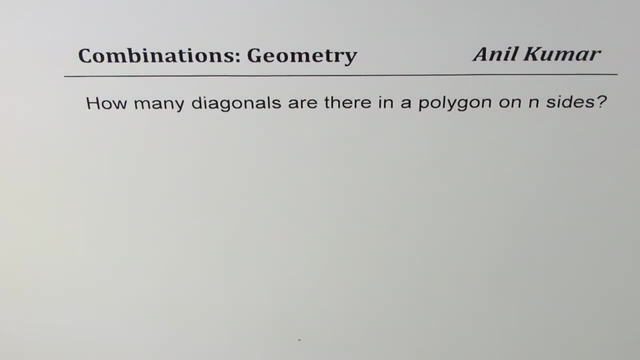 I'm Anil Kumar. We are exploring few cases where in counting the number of lines, we can use combinations principle. The question here is: how many diagonals are there in a polygon of n sides? See, if a polygon has n sides, that means there. 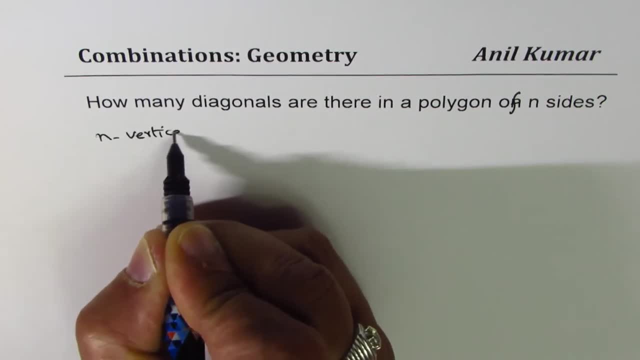 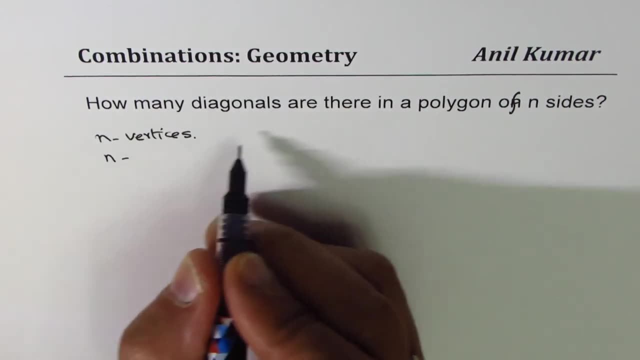 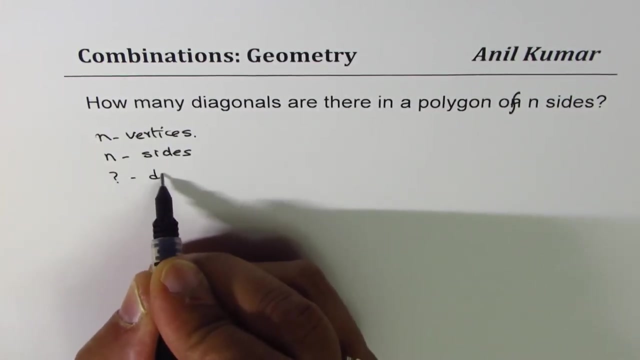 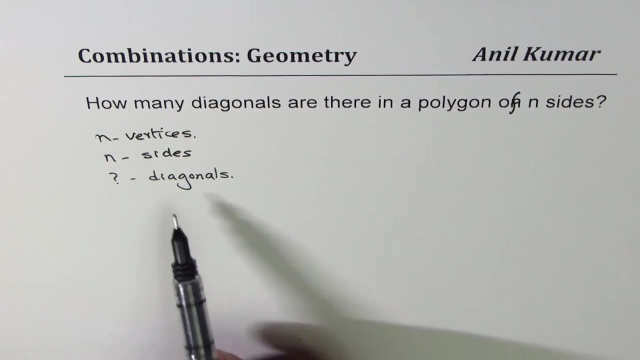 are n vertices, right, Correct? So how many diagonals are there? There are n vertices and there are n sides, Is it okay? So there are n sides And we want to find the number of diagonals, So that is the question. So the question here is how many diagonals are. 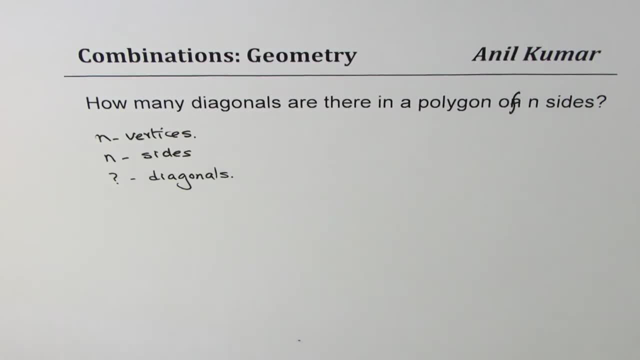 there in a polygon of n sides. You can always pause the video, answer the question and then look into my suggestion. Now, if there are n sides, we have n vertices, So we could consider n points scattered like this right And none of them. no two points, no, three points are collinear. That is very. 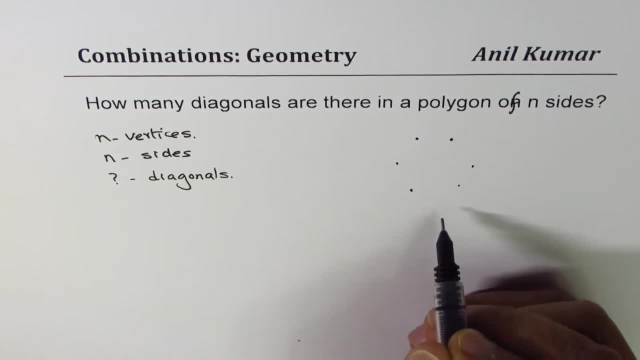 important when we talk about polygons, correct. Now, let us say this is a set of points In this case. we have a set of points. Now let us say this is a set of points In this case. in that case, the lines which we are talking about could be the edges, right. So I have. 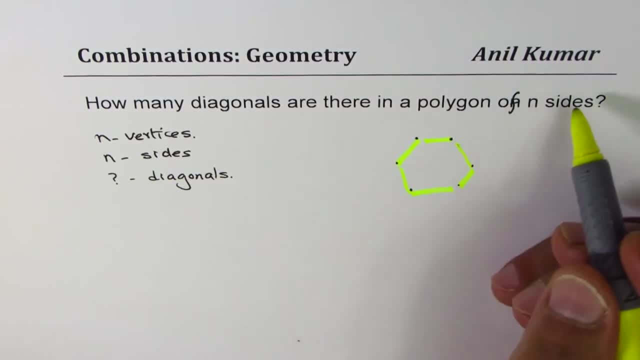 taken up an example where we have not n but limited 1,, 2,, 3,, 4, 5, 6 points, right. So we have 1,, 2,, 3,, 4, 5, 6 edges, So it is a hexagon right And we could also join with. 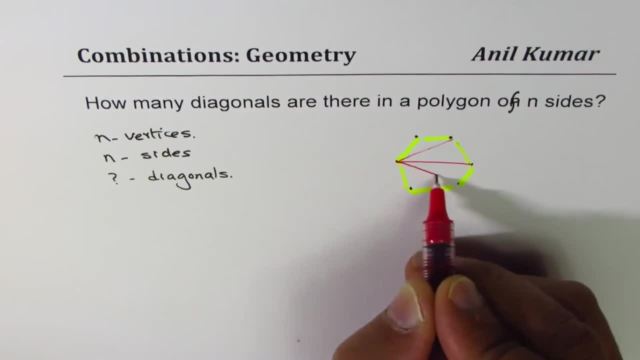 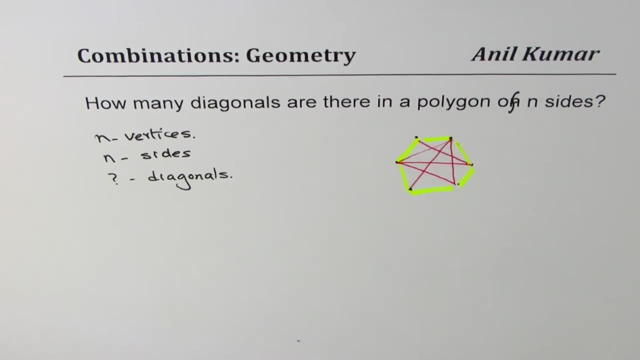 these lines which are called diagonals, Do you understand? so these are the diagonals we're talking about. so that is how you can make diagonals. so we want to know how many diagonals are there for n-sided polygon? I hope the question is absolutely clear. you can now pause the video and answer. 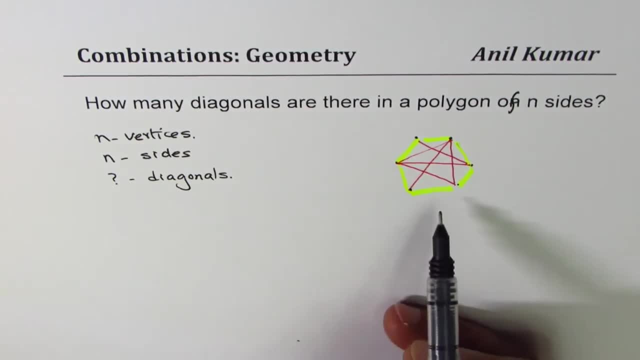 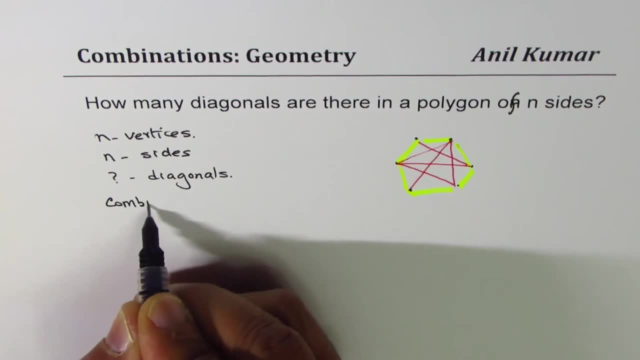 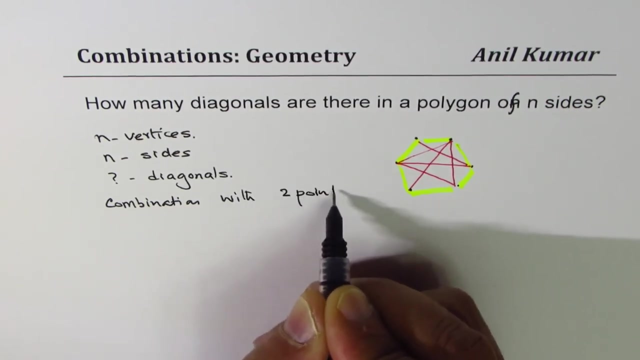 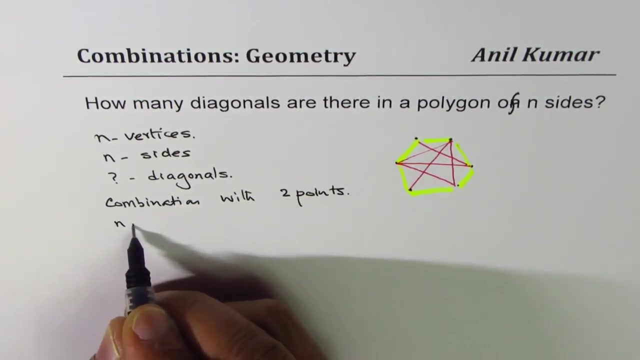 the question. right here is my solution: to draw a line, we need two points, right? so we're looking for combination with two points. is that okay? and how many sides or points we have? we have n points, so it is n. c2 is number of lines total. 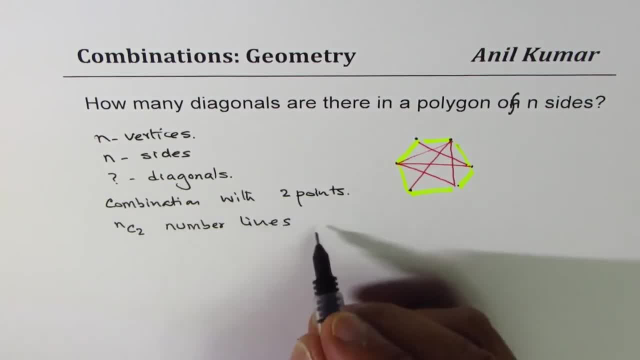 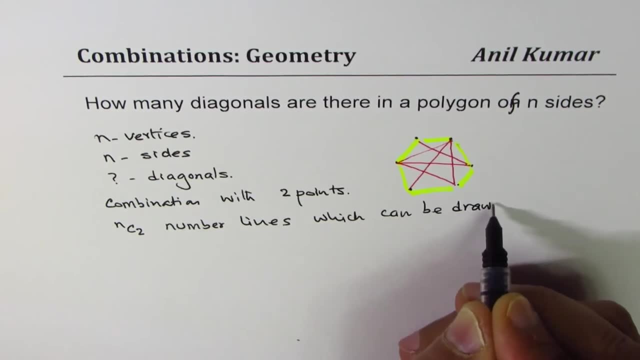 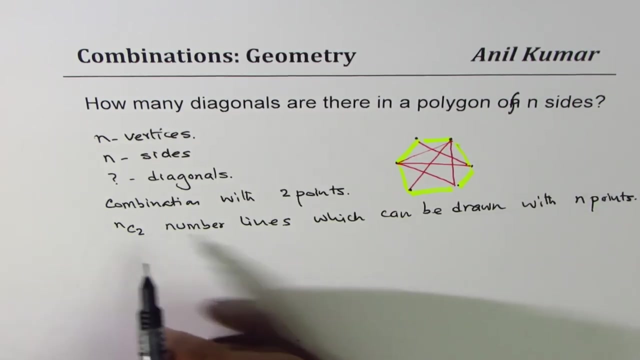 number of lines n, c2 is the number of lines which can be drawn with n points, correct? So out of these combinations you find how many diagonals? that is the question. So the diagonals will be total number of lines minus the edges, which. 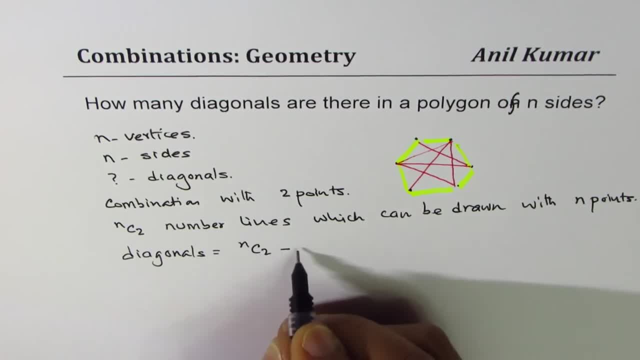 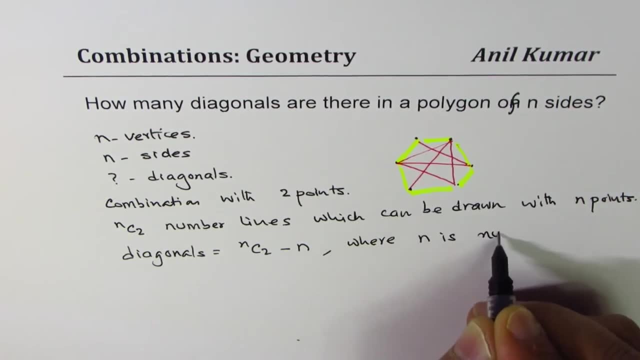 are n right. So diagonals are n c 2 minus n, Where n is number of sides correct. So that is how we get number of diagonals. So number of diagonals is n c 2 minus n. 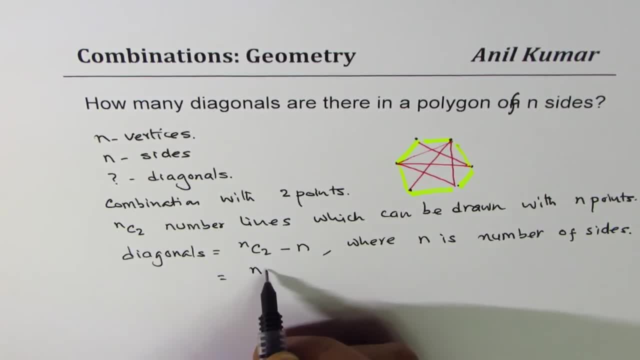 n c, 2, you write this as n times n minus n, 1 over 2, right minus n, and you would simplify this. if I open the bracket, we get n square minus n. multiply this by: we get minus 2, n, taking common denominator. 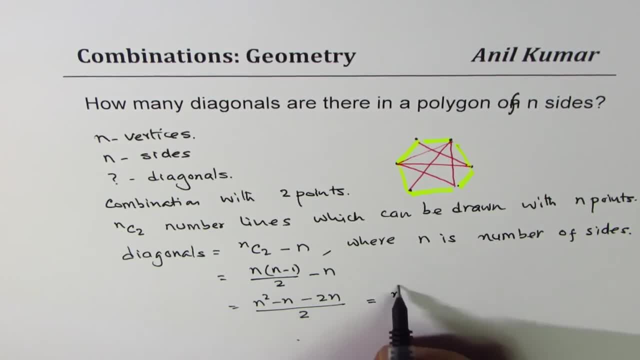 of 2, is it okay? so that gives us n square minus 3, n divided by 2. so that becomes a general formula to find number of diagonals. you get an idea right. so if I have a polygon with 10 sides, for example, or 10, I mean 10 sides in that. 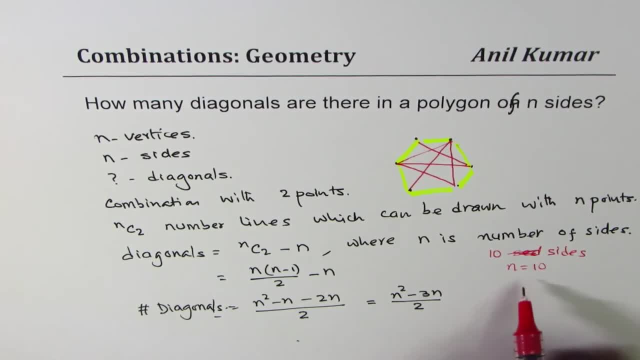 case n equals to 10, perfect, and the number of diagonals will be how many? let's calculate. so number of diagonals will be 10, 10 squared minus 3 times 10 over 2, right, So we can use the calculator.